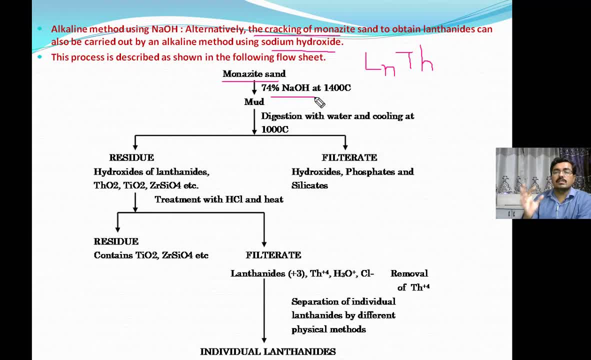 74 percentage of sodium hydroxide at 140 degree Celsius temperature. It is not 1400 degree Celsius temperature. The temperature is 140 degree Celsius temperature. So what will happen with that? We will get the paste of all the lengthenates in the monazite and thorium, So it is also known as mud. 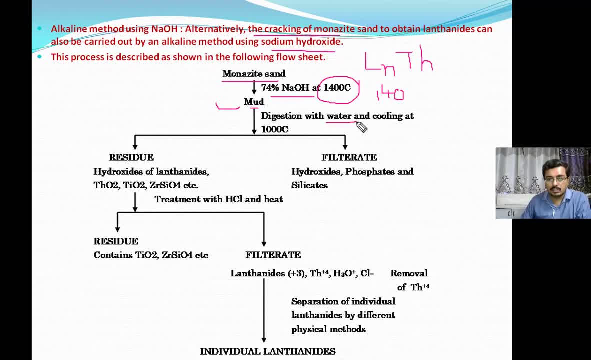 Now, in this we are adding a water and we are cooling it at 100 degree Celsius temperature. So the temperature here is 100 degree Celsius. Now when, in 100 degree Celsius, we will place it at temperature and diagnostime it, so that will happen. 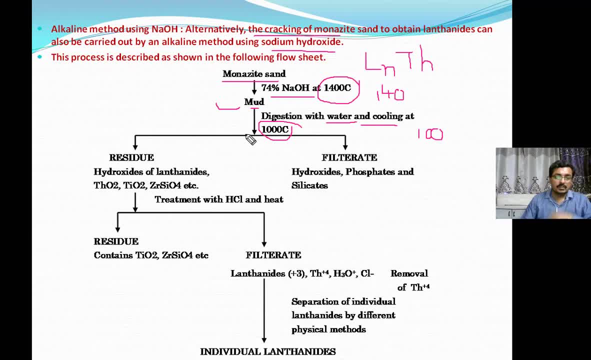 two thing. Insoluble mass can be a solid form, So insoluble mass will be obtained in the form of a residue. It'll be obtain in the form of residual, and soluble mass will be obtained in the form of filtrate, The way we're making tea. now this tea will sit like thatIt will, 수겐. with sugar, You will see that it will boil in a few minutes. As you can see, it has been subsided a couple of times, So it is getting bump tomorrow. So because we are getting meat and it is full of lye. 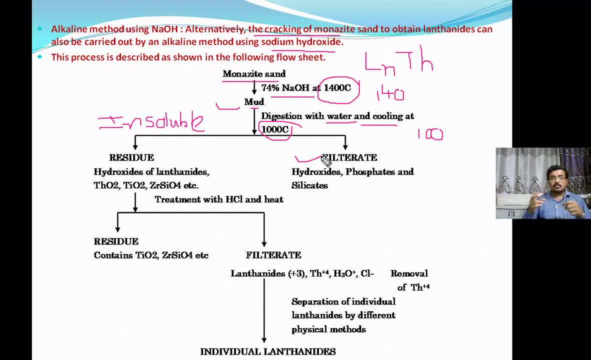 after that we will filter it with a funnel. so the solid mass, ie the powder of the tea, we will get it in the upper side. in the solid form we will call it insoluble mass means it is residue. we will get the filtrate below. 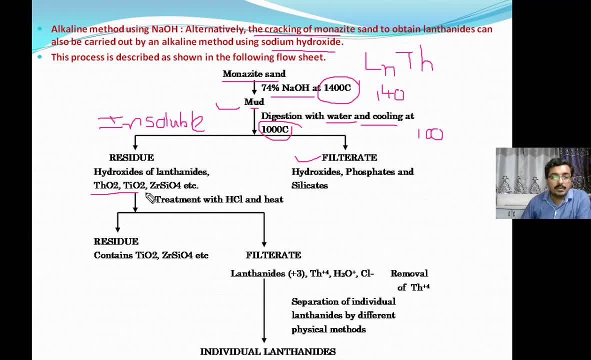 now what will happen is in the insoluble mass we will remove three impurities. which are the impurities? one is thorium, metal in the form of oxide. second is titanium dioxide and silica of zirconium metal. so in the residue, these three things are removed easily. thorium is removed. 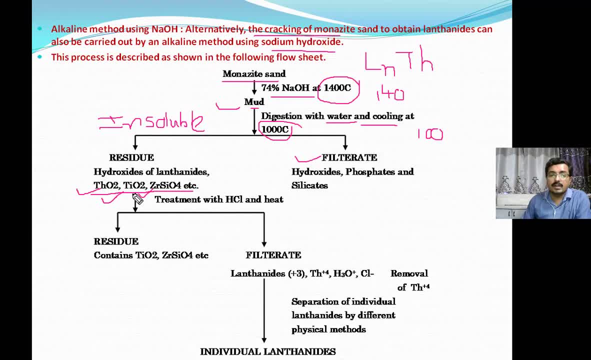 titanium is removed and zirconium is removed, and what will happen in the filtrate, the second metal other than the lanthanate? it has some hydroxide, phosphate silicate. we get it in the soluble form, so it will be removed in the form of filtrate. 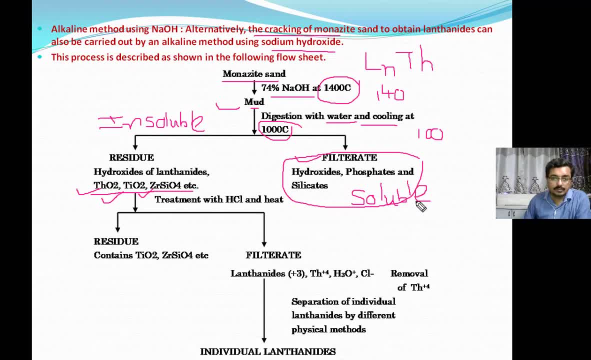 so first we will remove the soluble and insoluble mass. now this solid residue, we will treat it with HCL. as soon as we will treat it with HCL, we will get the solid mass as S and the liquid mass as L. so what will be removed in the solid mass? 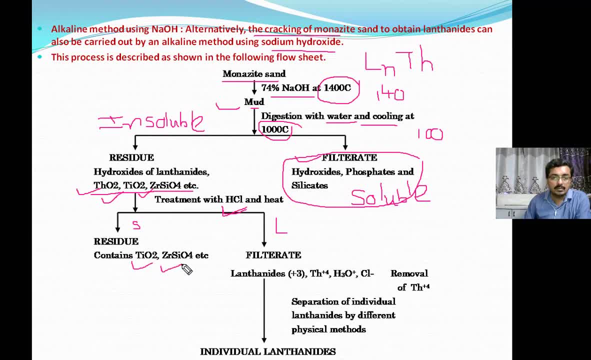 titanium will be removed in the form of dioxide. zirconium will be removed. here, the oxide of thorium will be removed. so by using this method, we will remove the solid mass from the solid mass and we have removed the three basic impurities present in a solution. 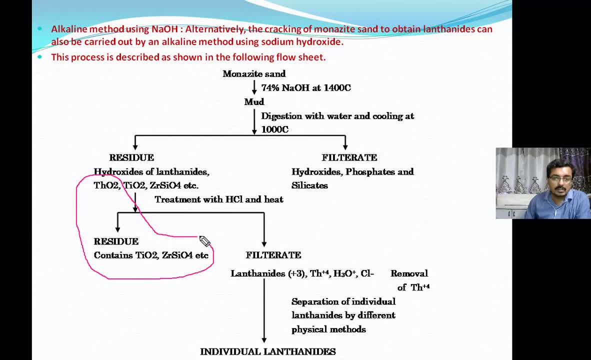 thorium is removed, titanium is removed and zirconium is removed. along with that, the silicates, phosphate and hydroxide of different metals are also removed. now in this filtrate, we will have lanthanate and thorium in the trace amount. now what will we do with this filtrate? 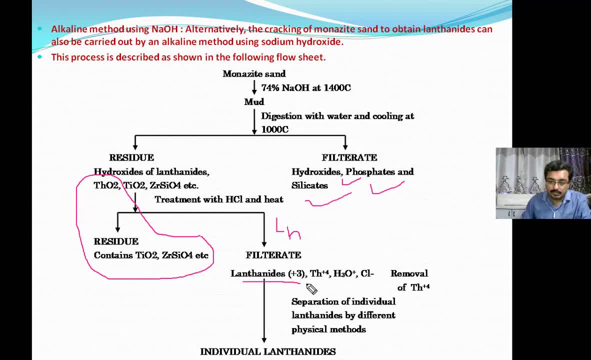 so in the filtrate we will have lanthanate with thorium and chloride, so we will use different methods to remove thorium from here. so after that, the liquid we get, this liquid having a lanthanate element, and this lanthanate element will be present in the form of chloride. 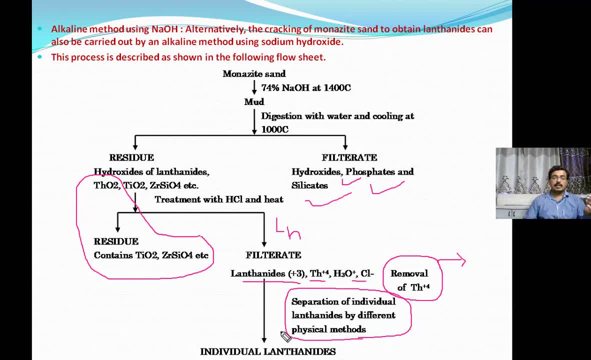 or it may be present in the form of oxide. so the chloride can be separated by using individual technique for each lanthanate element. so this is the basic method. by using base monazite mineral can be separated from it different components. so once again we will repeat the flow chart. 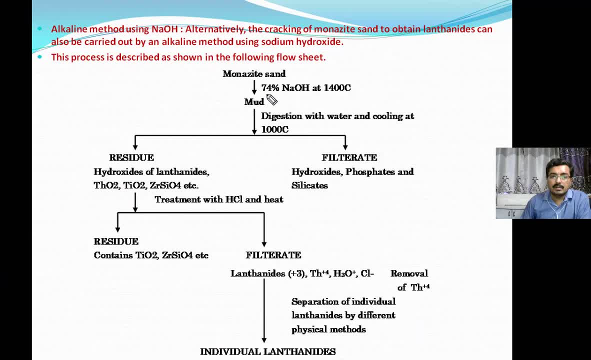 it is very easy and interesting. first we will take monazite 74% with sodium hydroxide. we will heat it at 140 degree celsius temperature. so we will get mud. that means we will get a paste. we will react that paste at 100 degree celsius temperature. 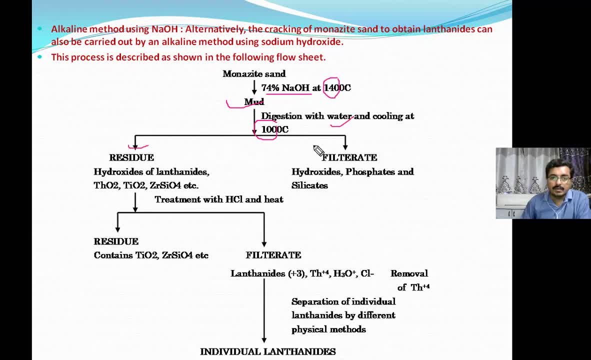 with water, so we will get residue and filtrate with filtrate. we have removed all these impurities. now thorium oxide, titanium dioxide, zirconium silicates and lanthanate hydroxide is present in this residue. we will treat it with HCL. 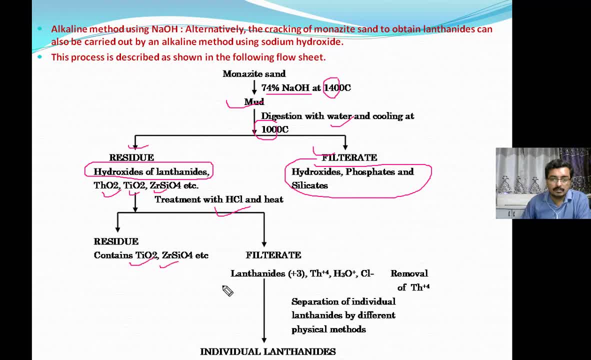 so these two are removed. titanium and zirconium: now lanthanate is in the form of hydroxide, thorium is in the form of oxide. so we will remove thorium, so we will get lanthanate, hydroxide or chloride. we will heat it. 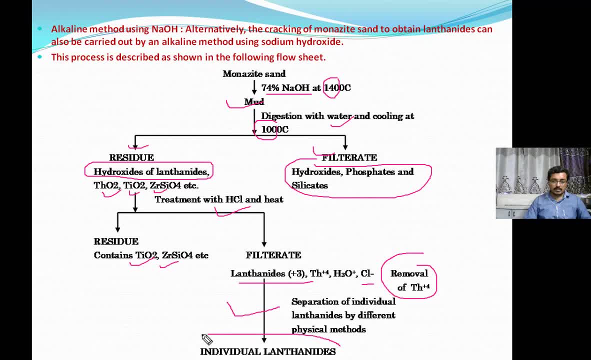 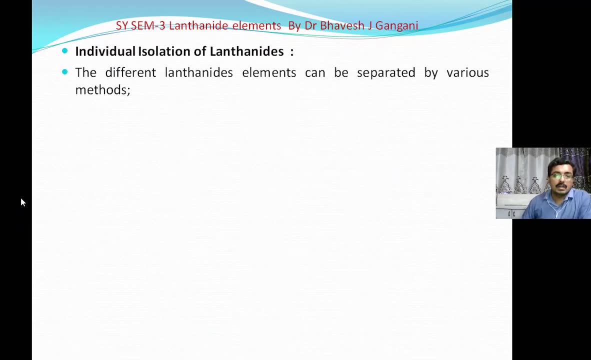 so it will be converted into lanthanate oxide and, using individual separation method, we can separate lanthanate. now let's study this individual method for separation of lanthanate. now. there are various methods for the separation of lanthanate elements. one of them is iN exchange method. 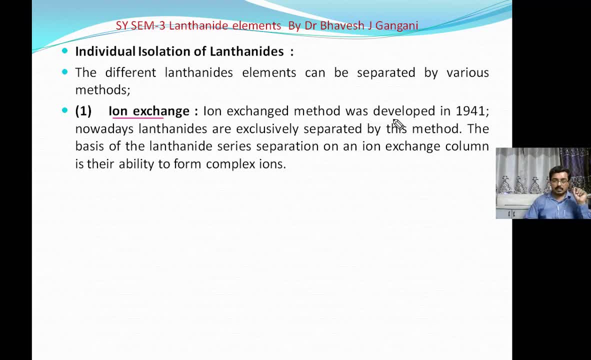 now this iN exchange method. whatever we are using for the separation of lanthanate element, each and every element can be separated by using a iN exchange method. so we use column for iN exchange method. I will take the next slide for you directly first. 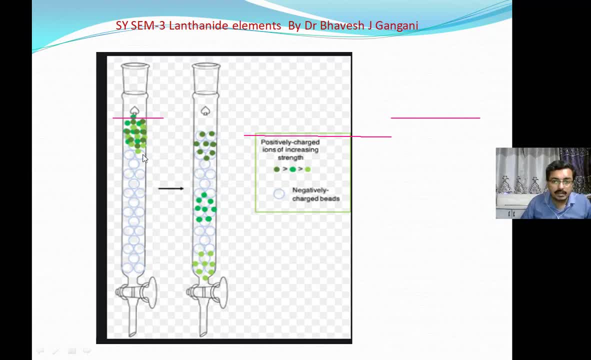 We take a column like this: We fill up in this column, which we will fill up in it. We have filled up the resin in it. It will be cation exchanger resin and it will be anion exchanger resin. We will pour the solution of lengthenate from here. 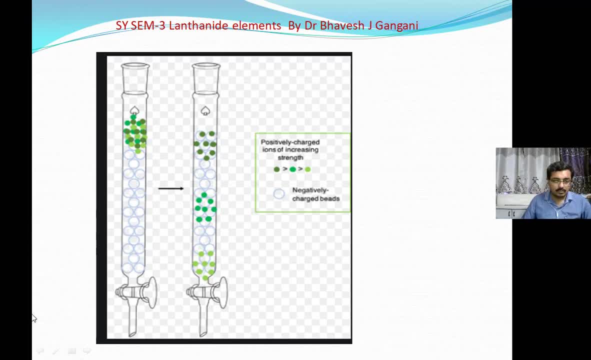 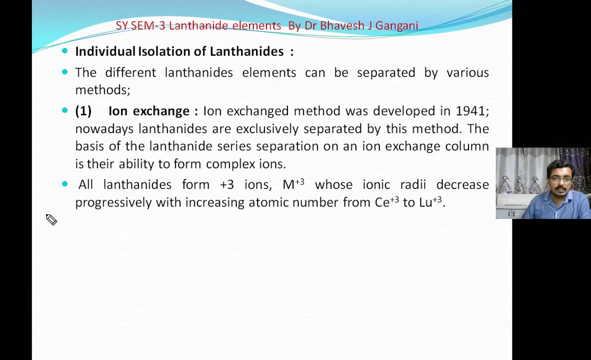 And we will pass it from here. When we pass, then from it Separation will happen. So now we go for this method. Now in lengthenate, Atomic weight is decreasing Because of lengthenate contractions, So we will get lengthenate, which is in plus 3 oxidation state. 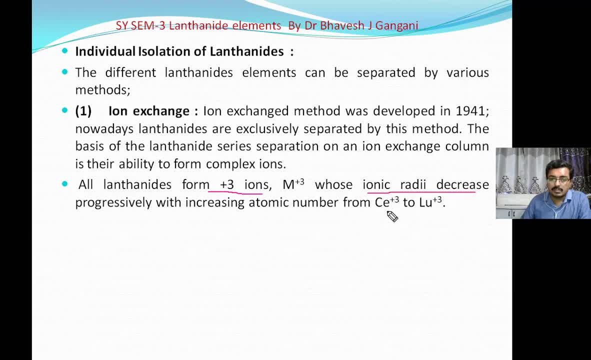 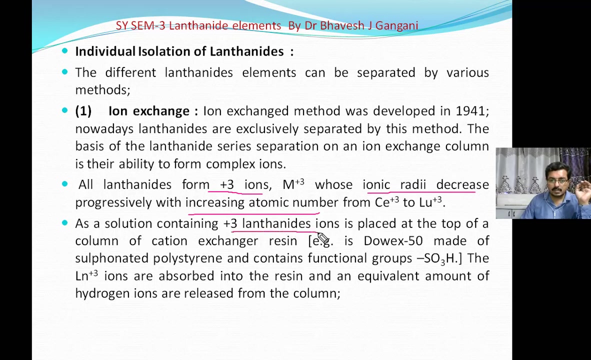 Ionic radius is going As we go from cerium to lutetium. Atomic size is decreasing with increasing in anion Atomic number. As the atomic number increases, The ionic radius of the lengthenate element is decreasing. Now what will we do? This plus 3 oxidation state. 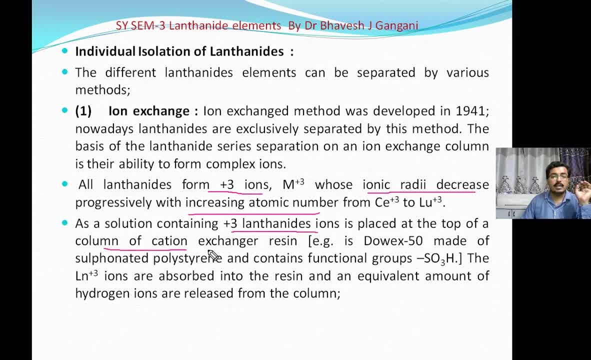 Which we have solution. We will Cation exchanger resin Now. we will pour in the cation exchanger resin. We will put in it. Cation exchanger resin is mostly sulfonate Or It has polystyrene functional group or carboxylic group. 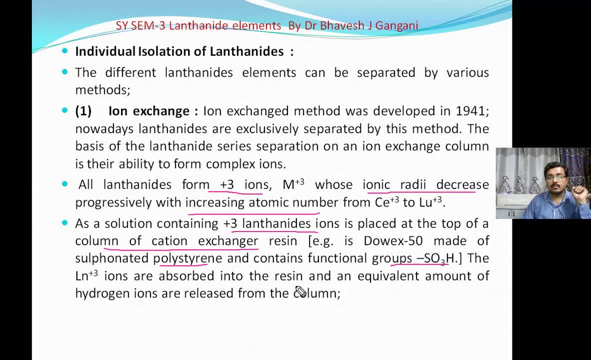 So what will happen in it? So the lengthenate ion will be absorbed on the resin And the carboxylic acid or the sulfate we have. Carboxylic acid has H Or The sulfonate has H, So H will be exchanged with it. Means. 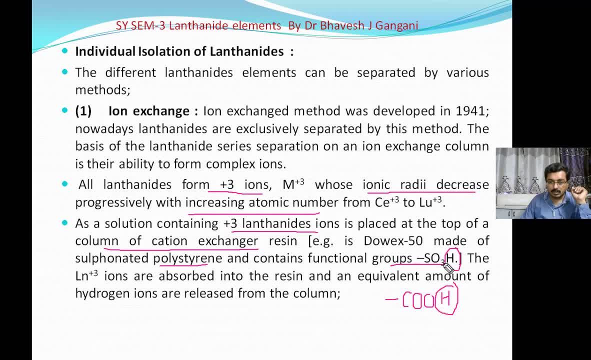 The lengthenate element is in the position of H plus And the H plus ion will go to the solution. So there is an exchange in it: H plus ion, Which is in the resin. They go to the solution And in the solution the lengthenate ion, Ln plus 3, goes to the resin. 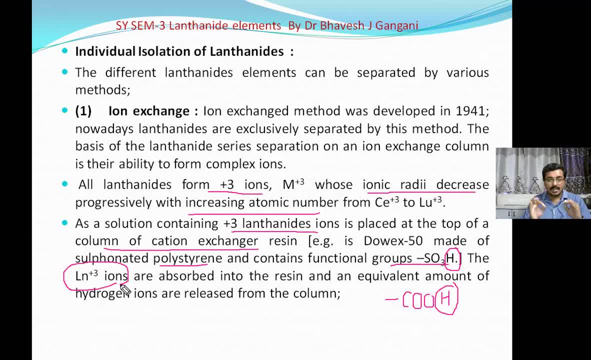 So in this The ion is exchanged. Then it is known as a Ion exchange method. Second thing: Here, exchange of ion occur Particularly positive ion Exchange. So it is a cation Exchanger resin We are using for this Method. So let's move ahead Here. we took cation exchanger resin. 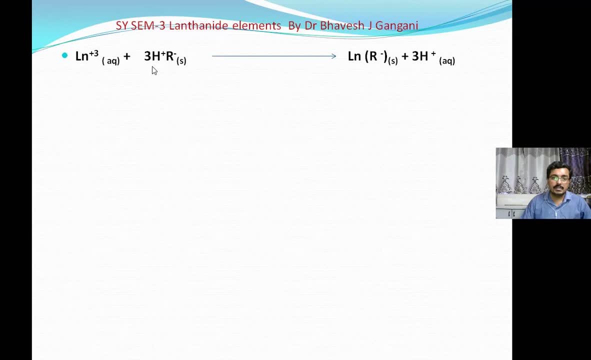 Pour it. So I told you that the H plus ion in the resin That Will go to the solution And the lengthenate in the solution will be attached to the resin. So this method is known as cation exchanger resin. Now we will use buffer solutions As the citric acid buffer solution. 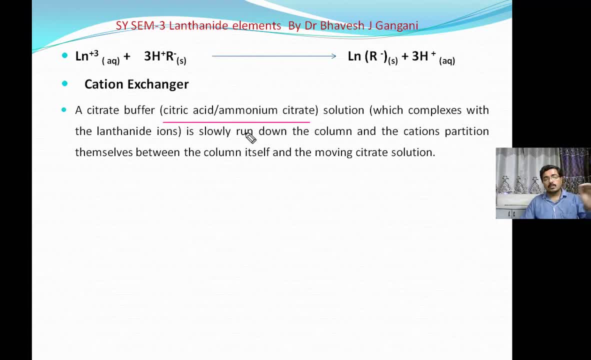 It is citric acid And ammonium citrate. We will put that In the column Above. So it is said that slowly, slowly, With this buffer solution, Cation will be coming And moving down in a Solution. So when we Put the buffer solution of citric acid in the column, 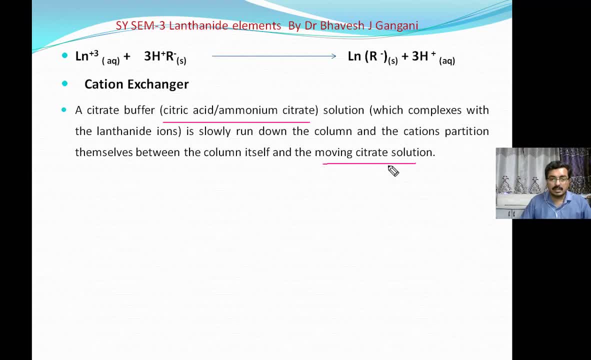 So the cation With the solution of citric acid. With the solution of citric acid It will move top to bottom. Now the small ion. It has a greater tendency to form a complex with a citrate Solutions. So in the solution the small size ions will come first. 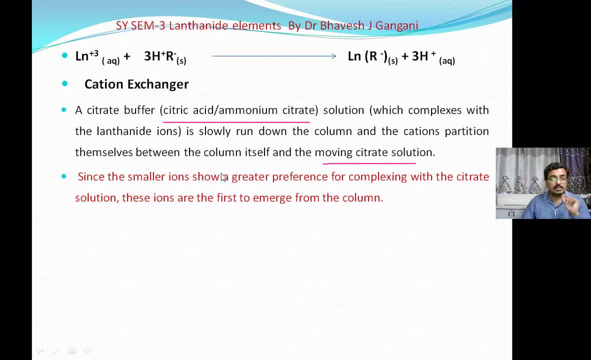 And the bigger size ions will come later. So why this happened? Particularly- I am reading this sentence again- The smaller ion having a greater Tendency or preference To form a complex ion with a citrate solution. So the smaller ion Will emerge from the solution first, That means in the solution. 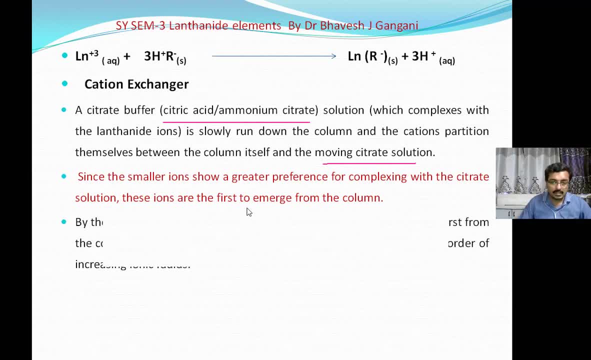 From the column, The smaller ions will come first. That means we will get cerium first. Sorry, Cerium's atomic size is Big, So we will get cerium at last And lutetium. We will get it first Because of lengthenate contraction as we move from cerium to lutetium. 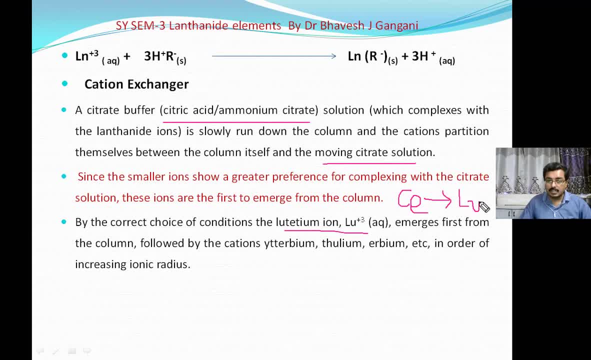 Or lutetiums. Atomic size of lutetium is decreasing As we go from Cerium to lutetium. Atomic size is decreasing due to lengthenate contractions. So First lutetium will coming out, Then after, At last, Cerium will Coming out. So according to, 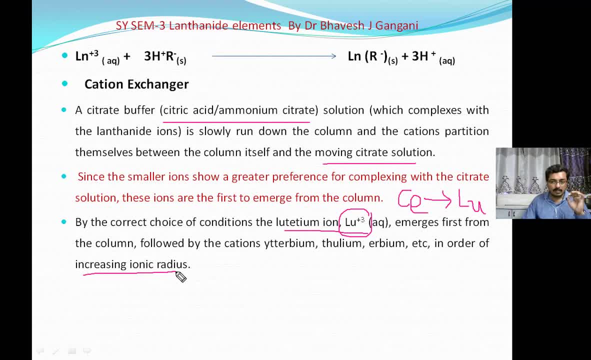 Increasing order of ionic radius, one by one, lengthenate element will come from Column. So now, By using this Ion exchange method, One can carried out 99.9% separation of lengthenate element. So this is the most important method, Easy method for the separation of lengthenate. 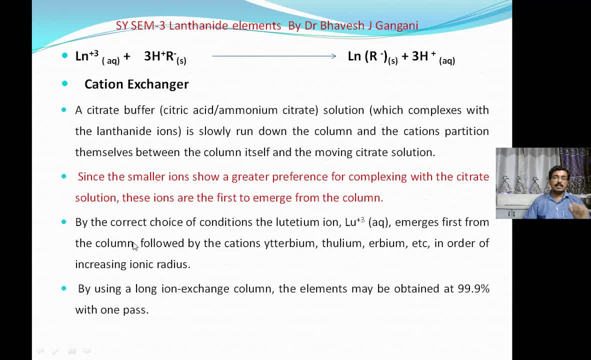 Element. Individual separation of lengthenate element is carried out by using ion exchange method Particularly. in ion exchange method we are using a buffer solutions, Buffer solutions. as a buffer solution, we are using a citric acid solutions. So citric acid solution with lengthenate element will form a complex 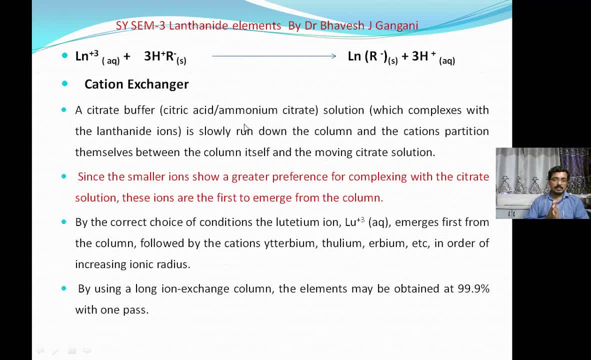 The size of the atom which is less than the size of the element will come first. So lutetium comes first And cerium will come At last. So, according to increasing order of ionic radius, lengthenate element will be separated by using a ion exchange Method. 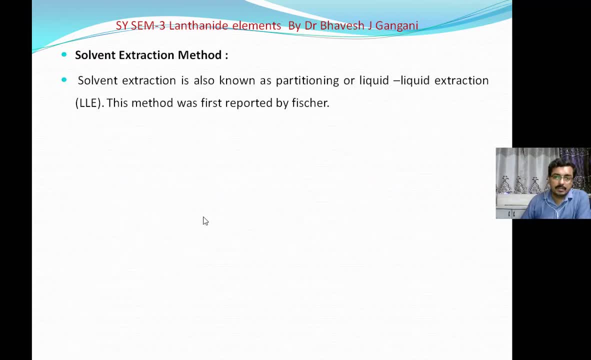 Now. Second method is a solvent extraction method. By using this solvent extraction method, one can separate the lengthenate element. This Solvent extraction method is known as a liquid Liquid extraction method, Or it was developed by scientist known as a Fischer, And Fischer has developed this method. Now this method is based on a. 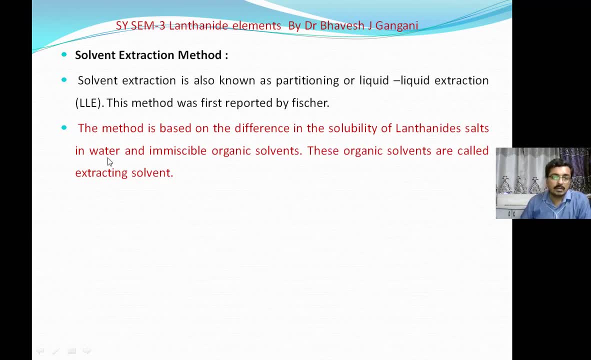 difference in solubility of lengthenate element in water, as well as in visible organic solvent. Lentenite element has difference in solubility. Lentenite element has different solubility in organic solvent and water On the basis of difference in solubility. this method has been established by Fisher. 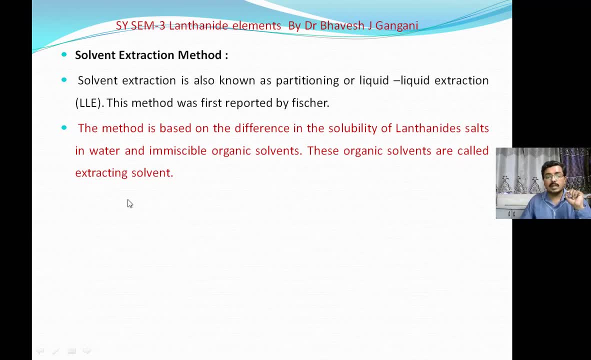 The solvent however we are using. it is known as extracting solvent. In this method, we can apply for tracer, amount or microscale separation. In this process, Lentenite salt: we are passing from organic solution With lented extract from water. This is aFilment and let me show you it's diagram. 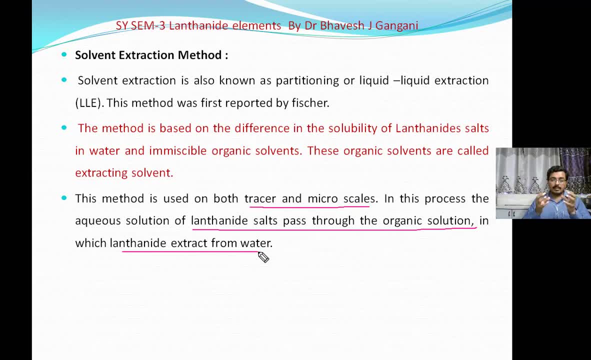 In that separating funnel we have taken organic solvent. In that we have taken the extract of lanthanate in water. We add that Now as an extracting solvent We will use TBP And the full name of TBP is Trinormal Butyl Phosphate. This we are using in an inert medium. 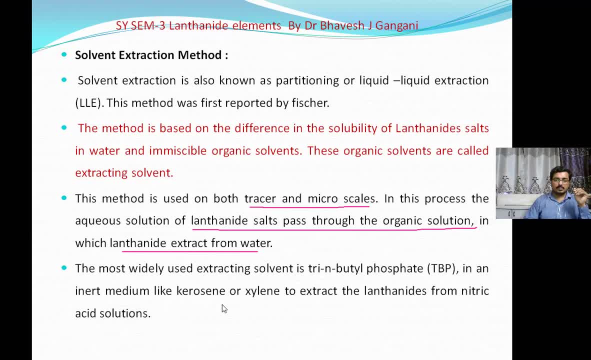 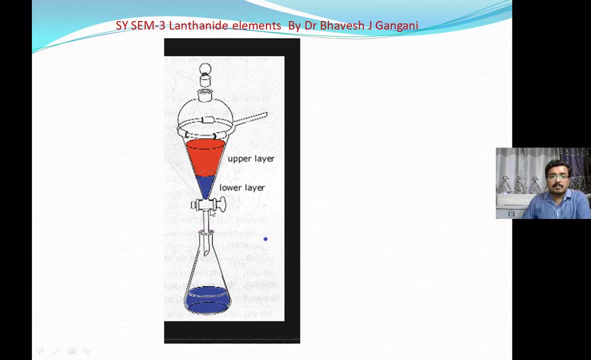 As an inert medium we are using. Gylene or kerosene can be used. Now lanthanate will be available in the form of extract. So what we will do When we have the extraction of lanthanate: We put the water extract in it And we will add the extracting solvent in it. 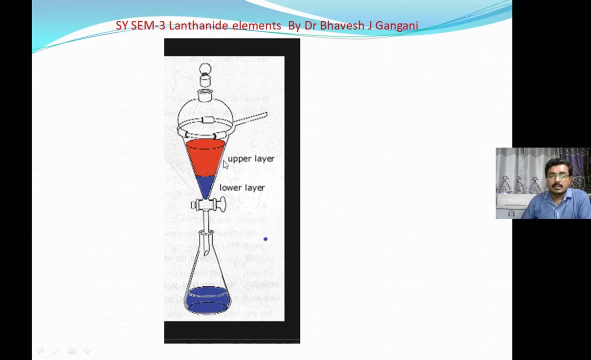 As an extracting solvent, we will use TBP. Now let's see The solubility of the lanthanate element in the organic solvent Will be high, Will be less in the water part. So what will happen From one solvent In the other solvent, Lanthanate element. 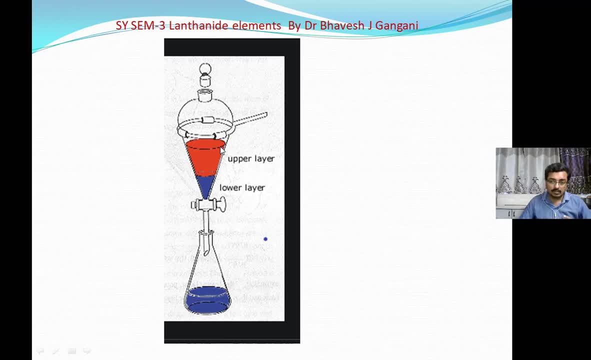 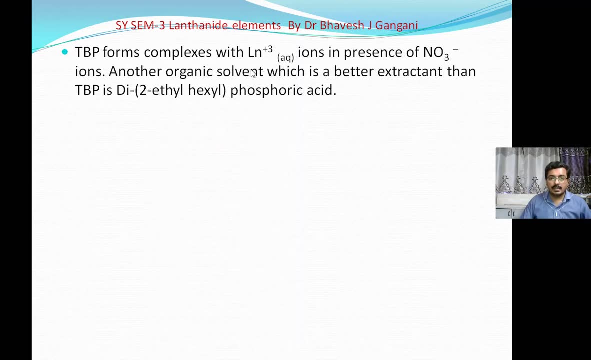 Will have migration. Then from that We can separate the solvent. So let's we go for What we have taken: TBP. We will make it complex with lanthanate. Now, other organic solvent Which we can use: It is 2-ethylhexylphosphoric acid.